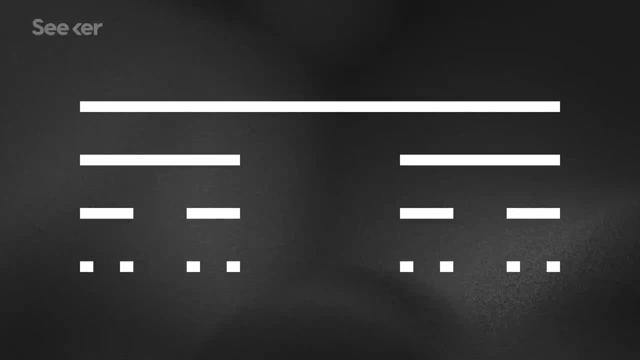 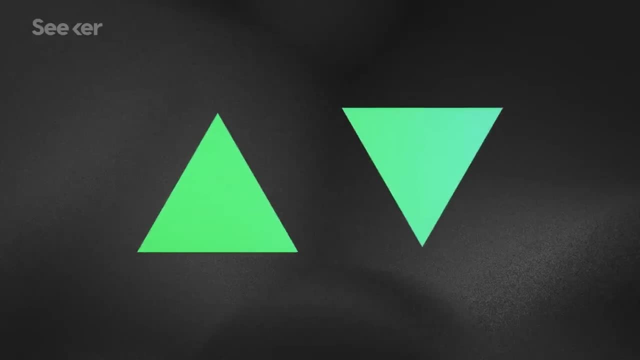 that same previous step, and on and on and on into infinity: a recursive pattern. But let's look at some more complex visuals. shall we Take the Coke snowflake? We have two triangles. We lay them on top of one another to make. 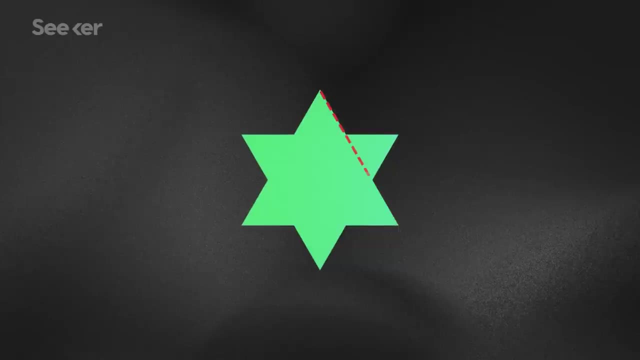 a star. We've taken each line of that original triangle and transformed it into four identical lines, each one-third the size of the original. That action can be expressed as a mathematical formula. Now we repeat that process and this is the recursive part, remember, with 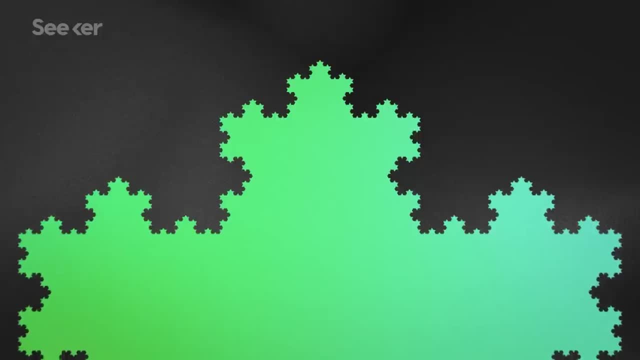 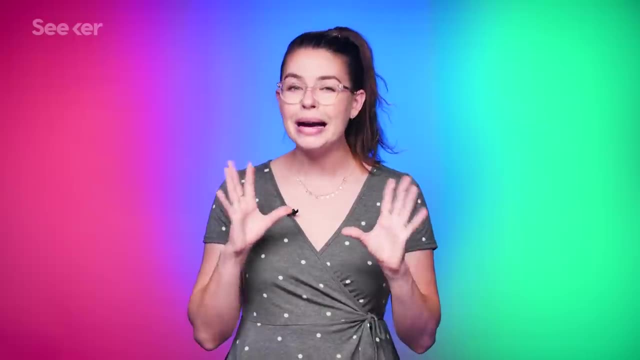 every resulting triangle, And so on and so on until infinity. Then every time you zoom in on a tip of the snowflake, you get something that looks exactly like the step before it. So the mind-blowing thing about the Coke snowflake is that the size of the object stays the same. 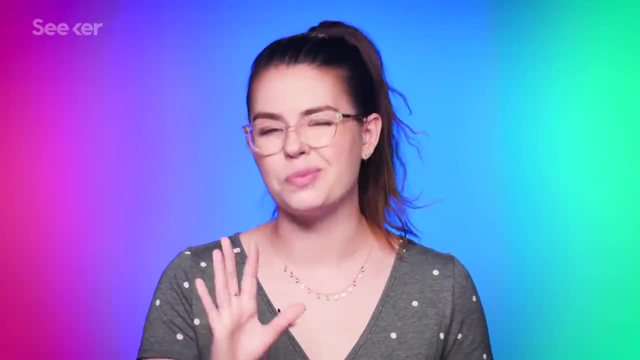 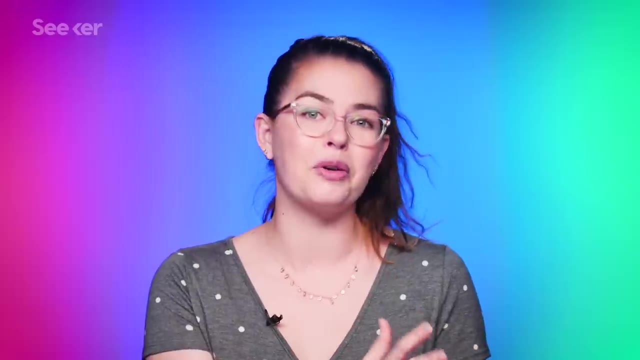 The snowflake isn't expanding as we perform this calculation, at least not significantly, but its perimeter is getting longer. In fact, the theoretical Coke snowflake has an infinite perimeter but finite area, which is so cool. Things like this are too complex for regular. 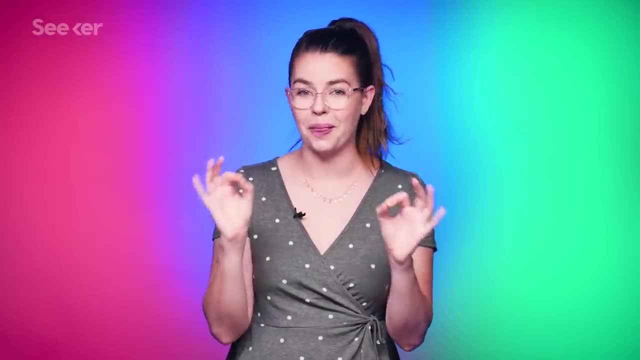 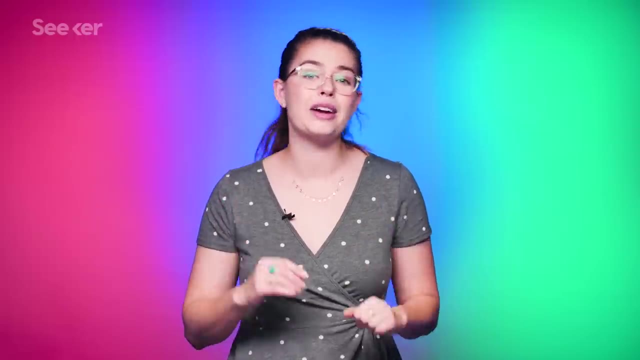 geometry, You couldn't take a ruler and go around and measure the length of each side of each triangle on the Coke snowflake. You would literally never finish, Which is why we have fractal mathematics that do work in this space. The resulting number from that. 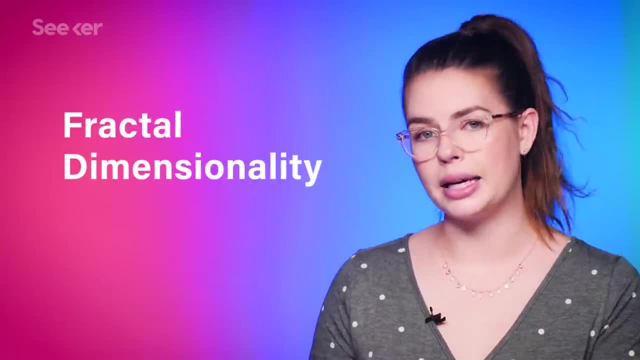 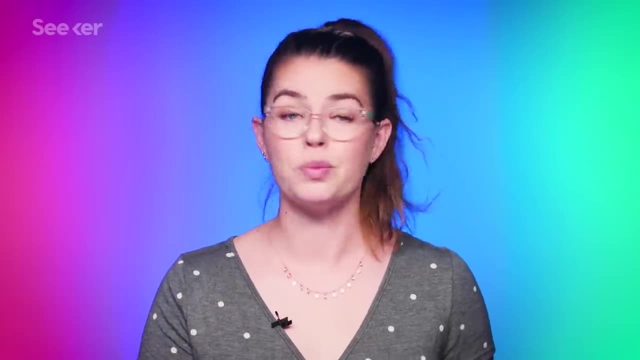 recursive equation is actually its fractal dimensionality. The Coke snowflake doesn't exist in one dimension and it also isn't quite two-dimensional. It's fractionally dimensional and has approximately 1.26 fractal dimensions. It's weird. I had literally 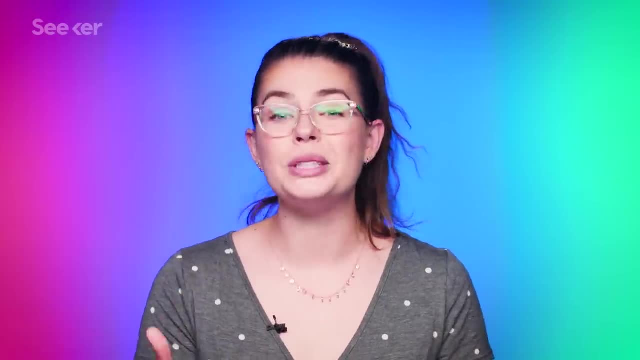 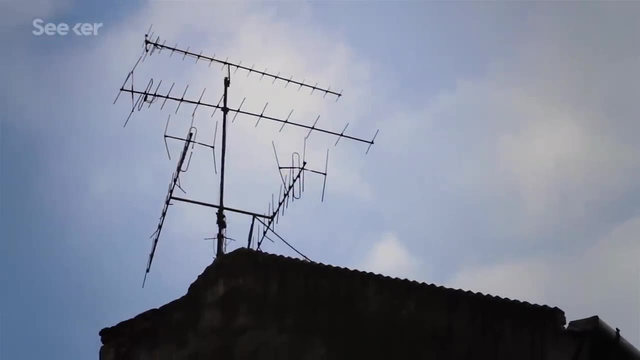 no idea that was possible. Alright, enough with the hypotheticals. What about real-world applications? For instance, we've applied the Coke example to the modern antenna. Regular antennas are designed to receive a certain range of signal types and are physically constructed to then. 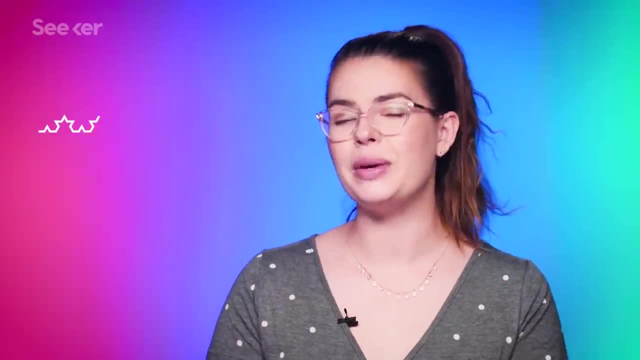 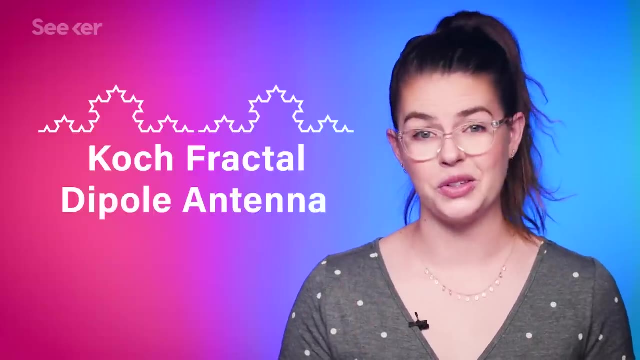 match that wavelength. But if we use some clever fractal thinking we can pack more shapes into a smaller device, making an antenna that is not only compact but can receive many more kinds of signals. We use the 3D version of this kind of antenna in our cell phones. 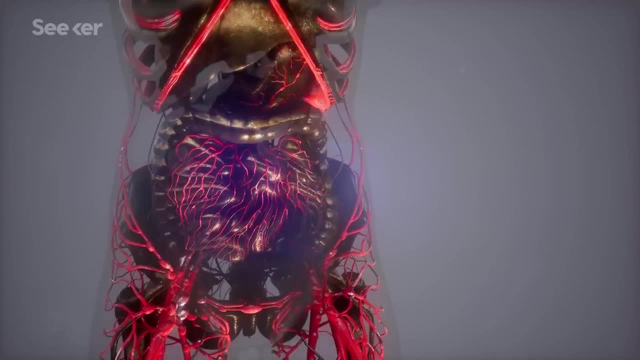 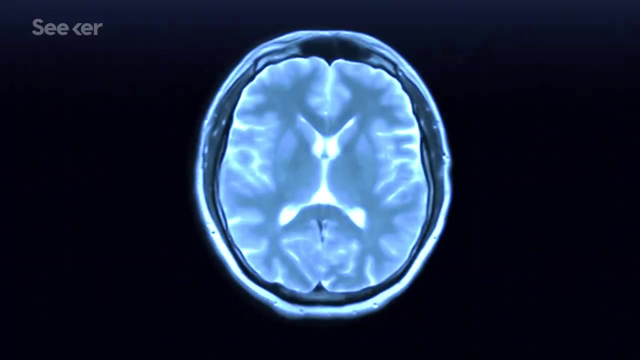 Fractal math helps us describe and model natural phenomena too: to make computer simulations of our circulatory and nervous systems, Or natural watersheds or brain waves, to better understand how all of these work And fractal patterns can exist, even on the molecular level, with really exciting results. 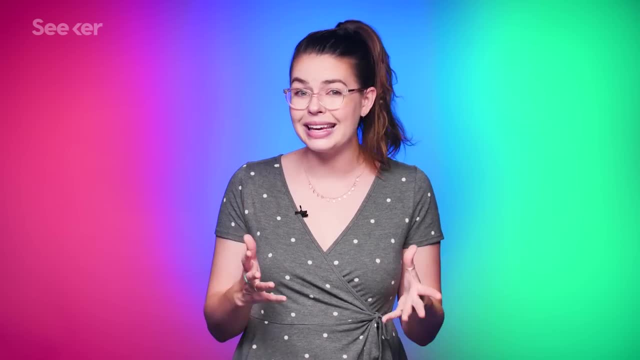 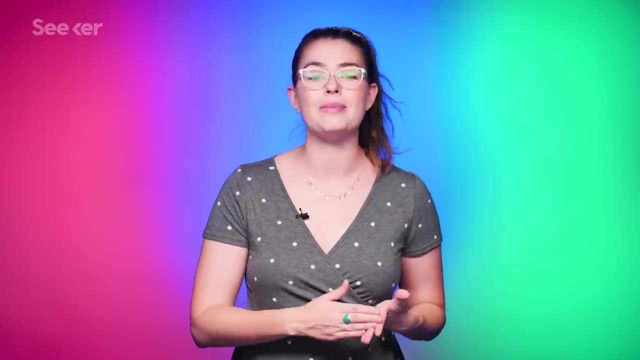 A new study has shown that researchers have been able to make and see a fractal out of electrons, specifically a Sierpinski triangle. To understand how this happened, we have to go back to the dimensionality of fractals. Electrons behave differently based on what configuration they're in, because of the 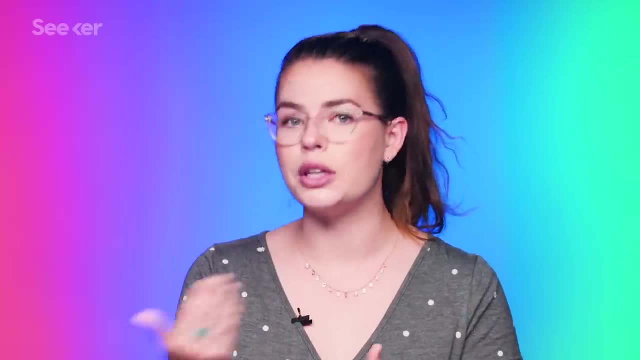 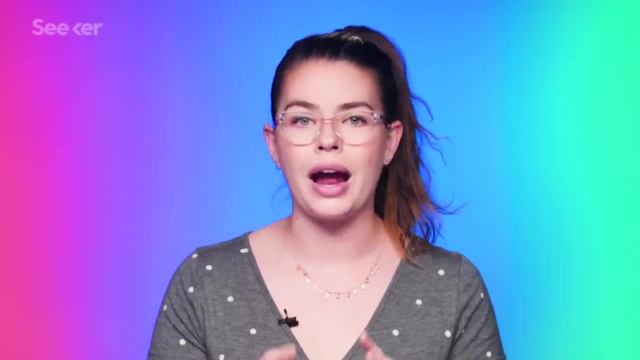 way their charges pull on each other. They're in one dimension, configured linearly, and in two dimensions, making up a sheet, or in three dimensions, in a cube. Their interactions with one another and their resulting behavior differs based on these configurations. 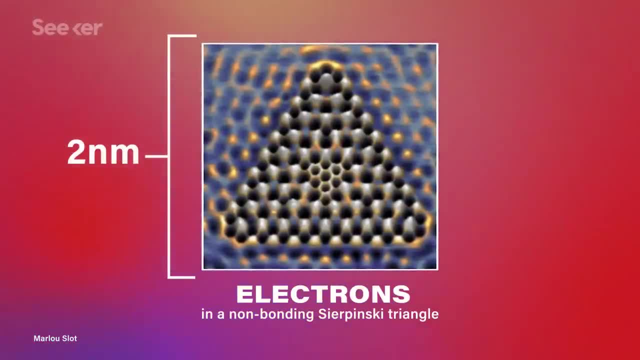 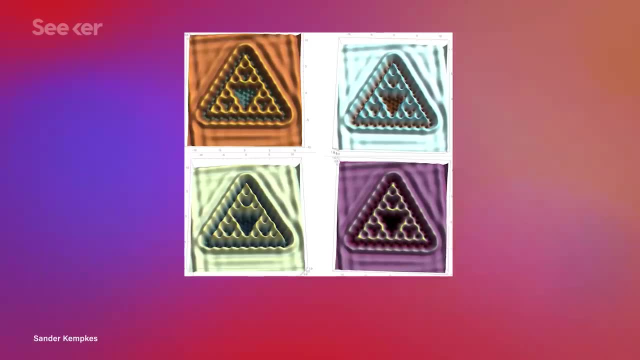 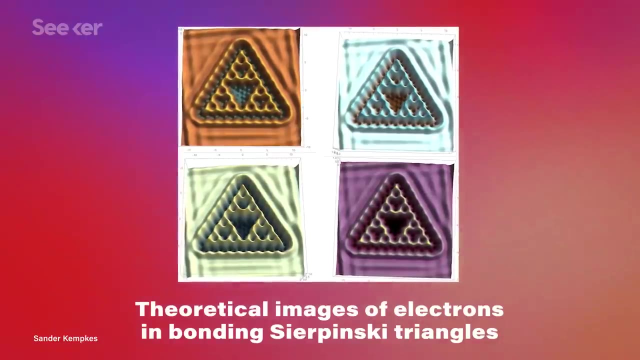 This team used a scanning tunneling microscope to place carbon monoxide molecules very carefully on a background of copper. The copper allows the electrons in these particles to behave very freely, so the measurements they took of the resulting shape, both spatial and in electronic wave function, showed that when in this shape the electrons behaved as if 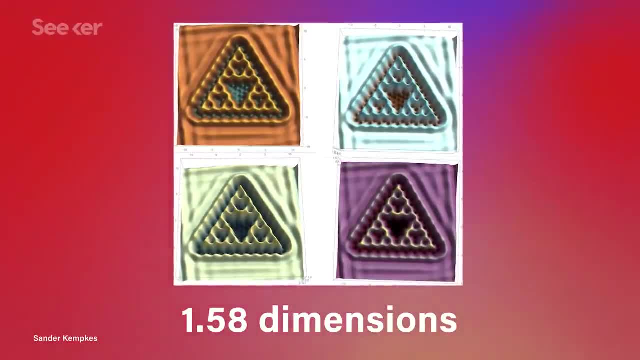 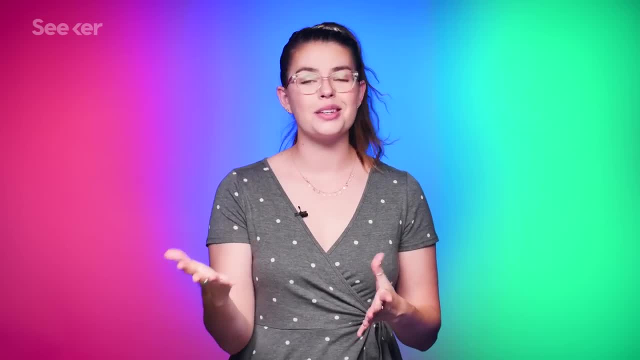 they were in 1.58 dimensions, the fractional dimension expected of a Sierpinski triangle: Teeny Sierpinski triangle fractals, just 20 nanometers big. The implications of this brand new research have yet to be fully explored, but we know. 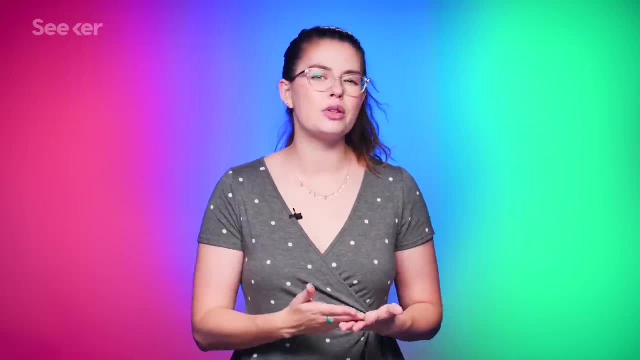 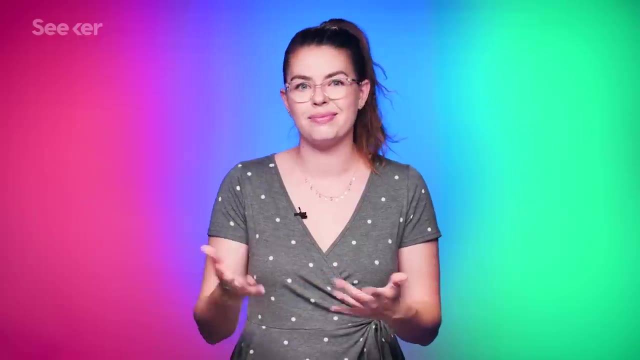 how useful fractals are on larger scales. so taking advantage of fractal geometries on such tiny scales could radically change the efficiency and versatility of our electronics, And it already has. Research has shown that if we employ fractal circuit elements, you can get a much. 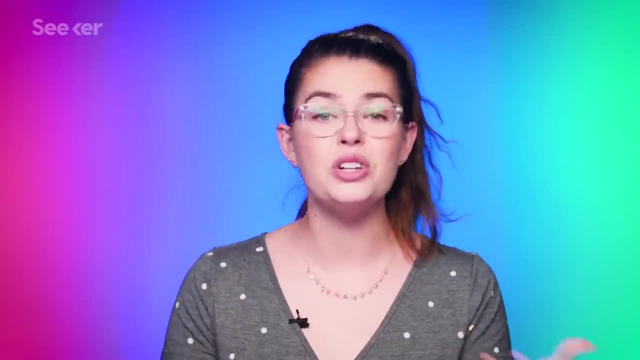 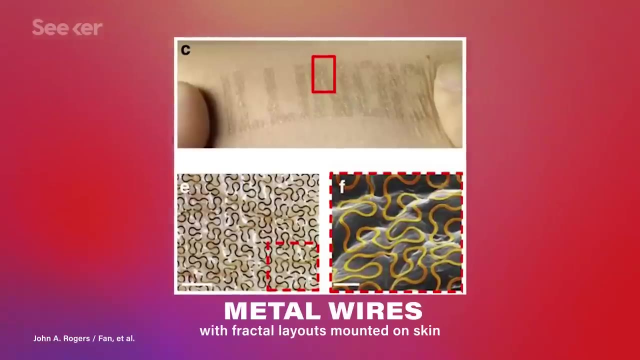 larger output signal, compared to the input signal, than you can with traditional circuitry. Or if we want to go even further out there, another team recently used fractal wire patterns to create stretchable electronics which you could wear on your skin. Okay, and just one last one, because it's so cool. 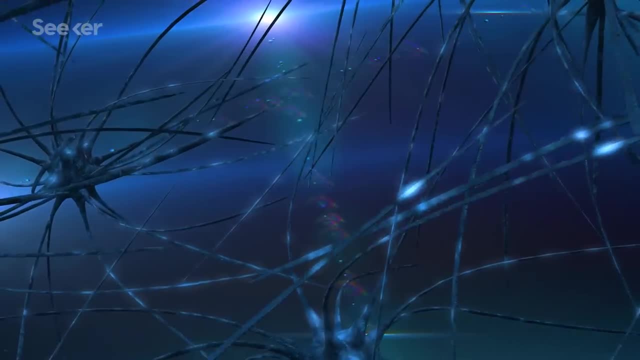 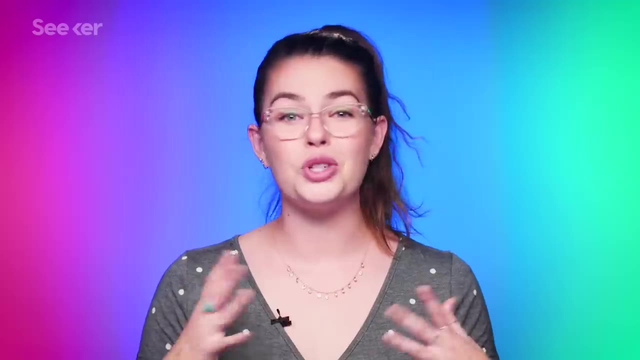 The neurons in our brain are fractal, which currently limits the applications of neural implants. But with fractal electronics, the bioelectric interface is something we could do a lot more with, Just like the fractal pattern itself. the possibilities here seem….